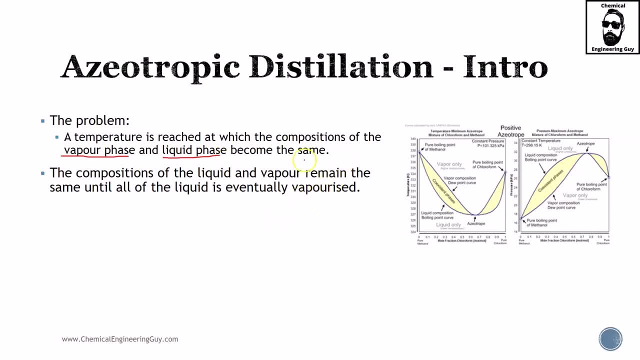 that this can be separated. This is the only point in which there is no separation between the dual and bubble points. The composition of the liquid and vapor phase will remain the same unless we change something, and that something is the main point of this lecture, guys. 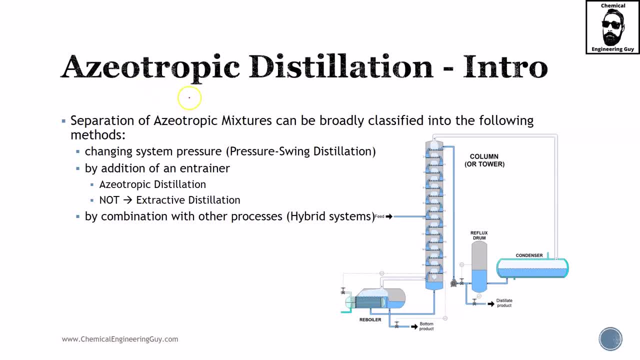 Azeotropic distillation is the main type of work for azeotropes, or trying to distillate azeotropes. Still, we can use distillation in such cases. and these are the three main categories. So first, changing the system pressure. 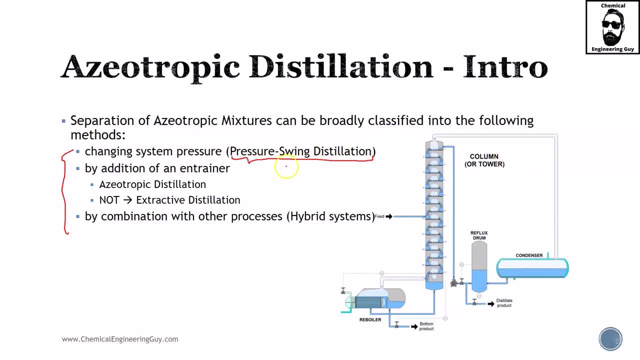 We have been talking about pressure shrink distillation, but this does not necessarily require us to have two pressure columns. You can do this by changing a single column. So, by definition, this will not be pressure shrink. this will be simply analyzing and changing the pressure of operation of the column. 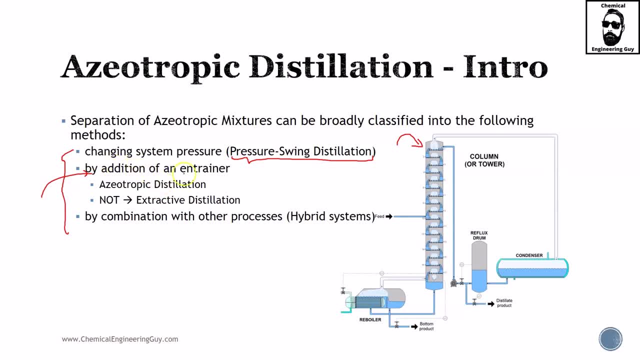 The most common ones will be by addition of an entertainer, which you will have- azeotropic distillation, the main focus of this lecture, And we also have extractive distillation, which we are not going to focus in azeotropic distillation because in this specific case, we're going to be working towards extraction. 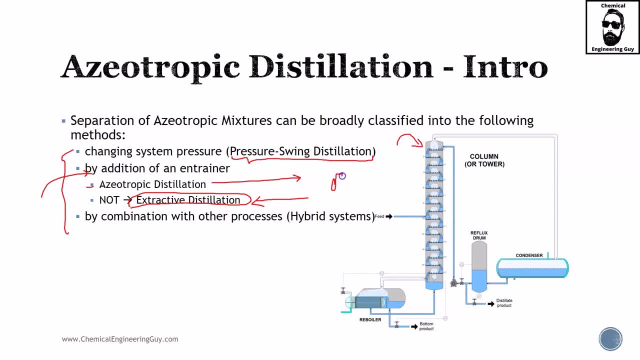 and in azeotropic distillation, typically we work towards the separation or changing that point and eventually recycling the entertainer, while in the extractive distillation we're going to be focusing on extraction. Make no worries, I am going to show you specifics on azeotropic distillation, on extractive: 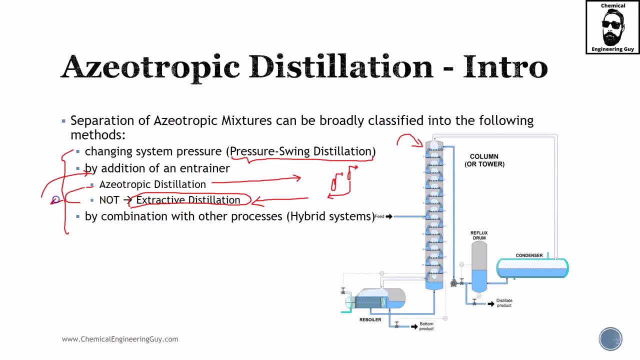 distillation and later on, a lecture which makes the main differences and similarities on these two main processes in distillation. The third category will be a combination of several processes, A hybrid system. A hybrid system: Either you use distillation, then you use membranes and recycling, or you use distillation. 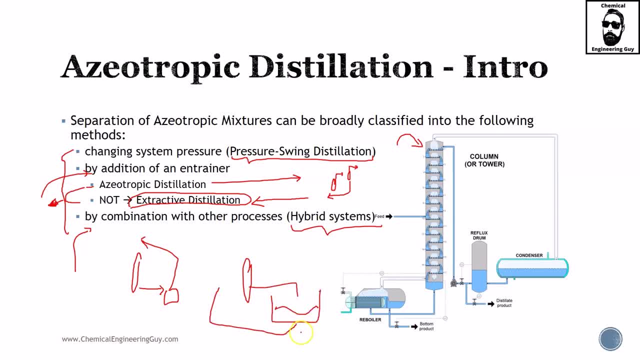 and then you use extraction and so on. There are many ways in which you could actually add several separation systems, the so-called hybrid systems, in order to solve the azeotropic distillation. We're going to cover azeotropic distillation first, which is the main case in which we